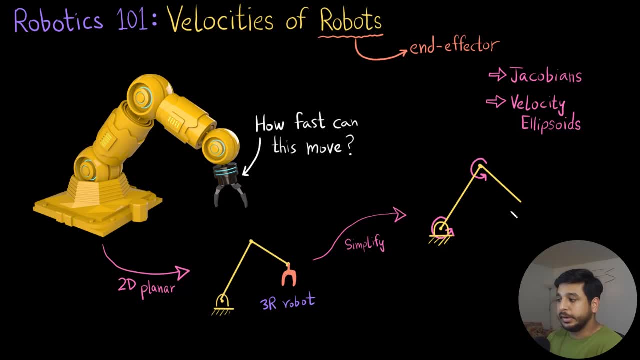 And at the end I have gotten rid of the end effector. And so now what the question becomes is what would be the velocity of the tip of the robot, which is the velocity of the end effector of the robot I have marked here. So I have to find out what the velocity is going to be of the tip of the robot. 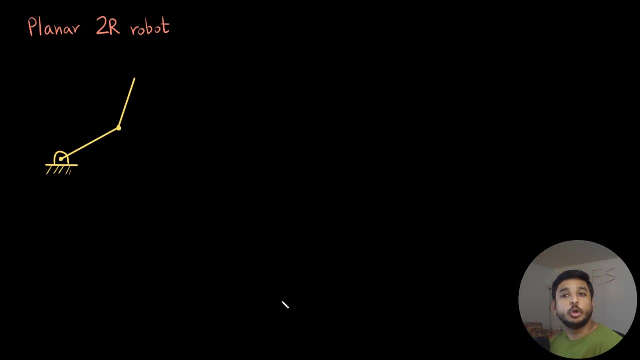 Now let me draw this robot again. So drawing this planar 2R robot again, and I know that it has got two revolute joints, one here and the other one here, So it has got motors at these two joints. Now, marking out the fixed frame. 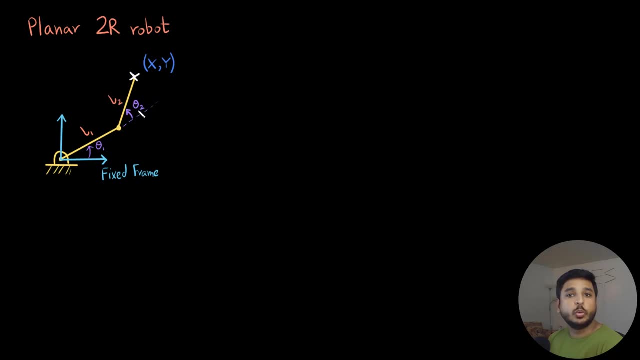 so this is my fixed frame right here. Theta 1 and theta 2 are my joint angles and a1 and a2 are my my dick dance, and this cross represents the tip location of this robot, with x and y being the tip coordinate. so the way i proceed with this is i do the forward kinematics of this first. so i've got. 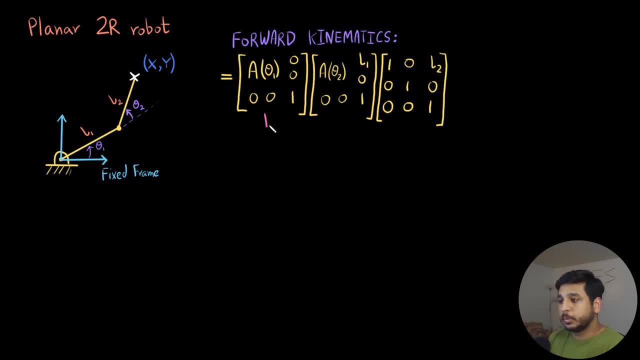 these three homogeneous transforms. i can call this as my h1 homogeneous transform, this as my h2 and this is my h3 homogeneous transform, where i know that a18- this term right here, is just this, which is cosine theta, sine theta, minus sine theta and cosine theta. so this a of. 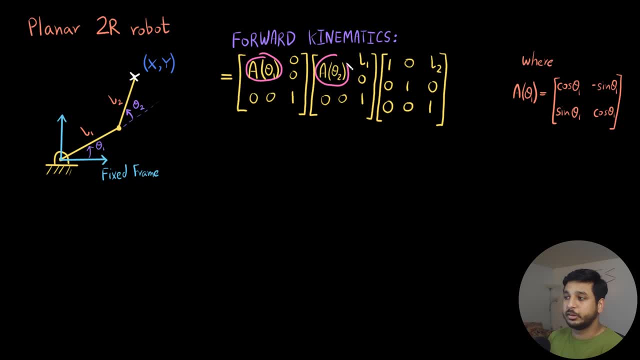 theta 1 is a 2 by 2 matrix and a of theta 2 is a 2 by 2 matrix 2, and if i multiply these three homogeneous transforms i get this where this again is a 2 by 2 matrix similar to this one. 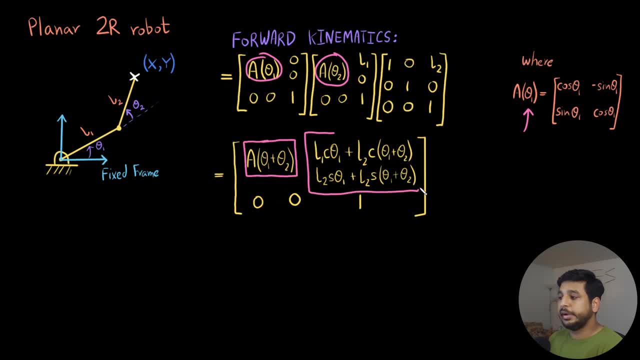 and these two terms that i get right here, if you remember that these two terms represent the displacement of the final frame. so this, what these two terms represents, are the tip location. so this, these two terms, represents the tip location, with the first one being the top one. 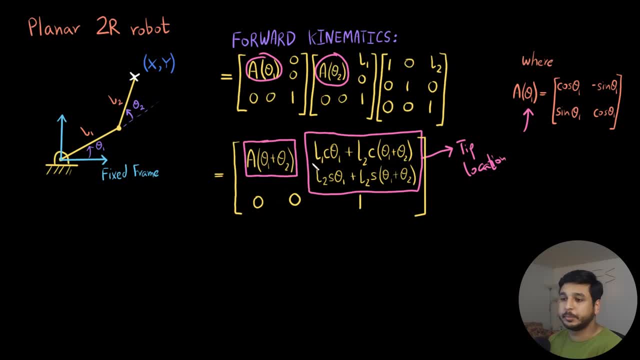 being the end point x coordinate and the bottom one being the y coordinate, if i go further. so i just i am just examining the displacement term of this forward kinematics right here, so i have just extracted this, these two terms, and written them in a slightly different form. so i've extracted a1 here. 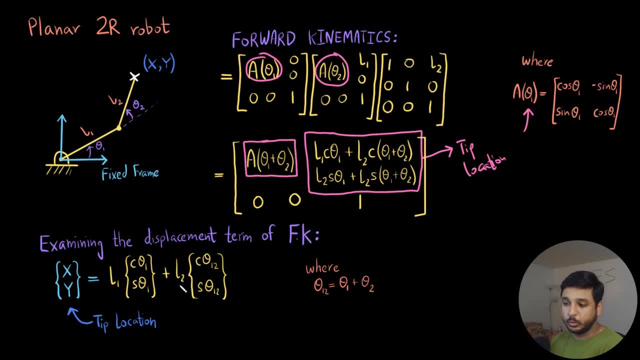 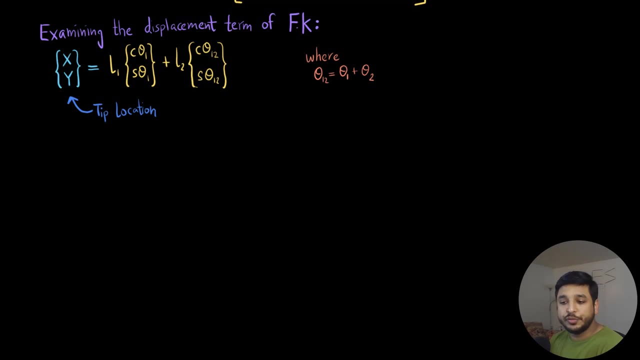 taking it out as common, and here i have taken out a2 and i have written theta 1- 2, which is the sum of theta 1 plus theta 2. now, in order to find out the velocity, all i need to do is i need to differentiate this. so, differentiating this, i get the tip linear velocity, which is just x dot. 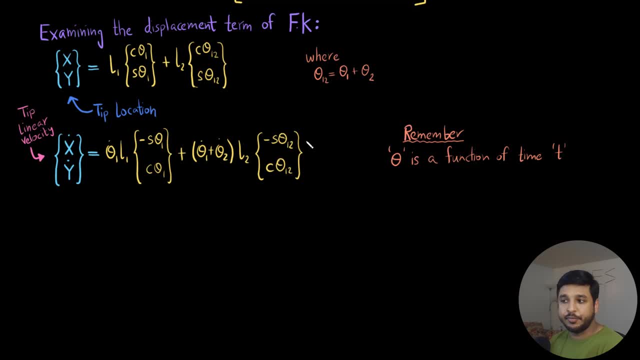 and y dot. and if i do the differentiation i end up with this and just remember that theta 1 and theta 2 both are functions of time. so when i take out the derivative of theta 1, i get theta 1 times theta 1 dot. 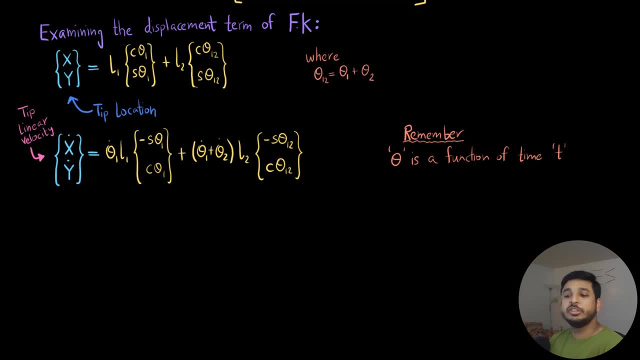 so i end up with this now. i just rewrite it another way as this: so what i have done is i have factored out theta 1 in this and made a bracket and kept everything to one side, and then i factored out theta 2 and i have made a bracket and multiplied everything that is being multiplied. 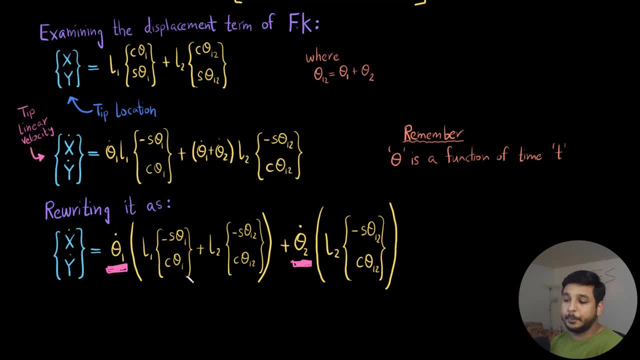 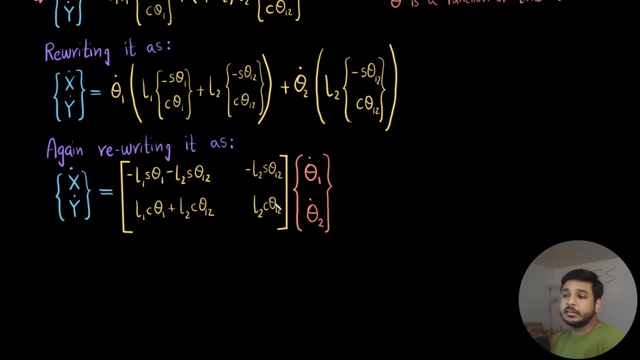 with theta 2. so i've got these two big brackets- one is for theta 1 right here and the other one is for theta 2. now i am going to rewrite it another way. just bear with me. so again rewriting this. so now i have rewritten this in another way. what i've done is i have just extracted theta 1 and theta 1 dot and 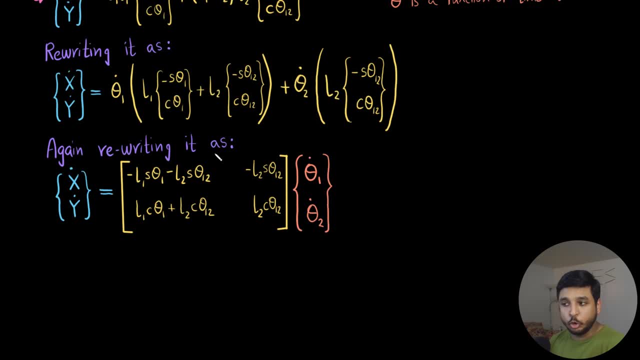 theta 2 dot in this way and i have made this a 2 by 2 matrix which is being multiplied with these, and on the left hand side i have the tip linear velocities. so just having a look at it, i can see that this one right here is my end effector space, which is just the velocity of 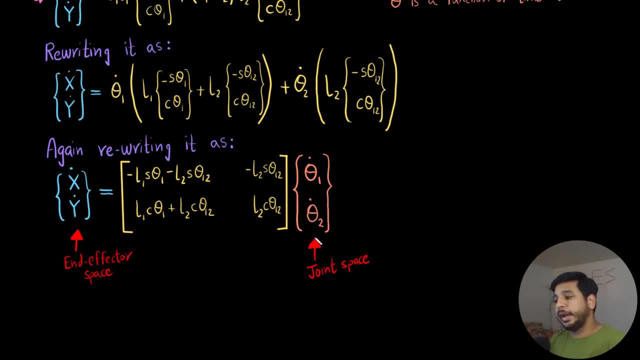 the end effector, so it is called the end effector space. and this on the right. this matrix, which is theta 1 dot and theta 2 dot, represents a joint space, since these represents the joint the, and the x dot and y dot represents the end effector. this equation shows me. this equation right here. what? 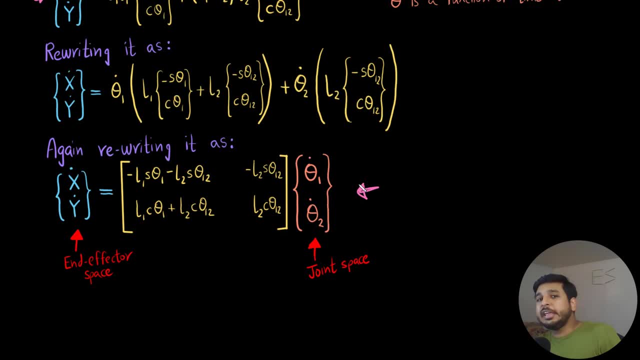 this shows me that if you were to give me any joint angle velocity, so if you were to give me, like theta one dot and theta two dot, i can simply multiply it with this two cross, two matrix and i would get the tip velocity in this matrix right here, which is the two cross, two matrix. you can see that this 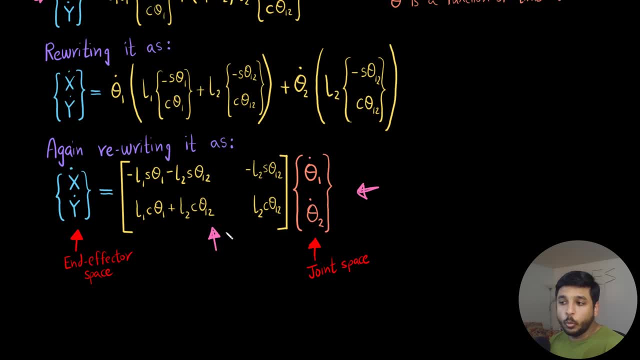 two cross, two matrix is dependent on two things. one is the link, dense, which, if you already have a robot, the dense are going to be constrained, so a1 and a2 are just going to be constant. and the other thing is it depends on the specific position of the robot at that particular instant. 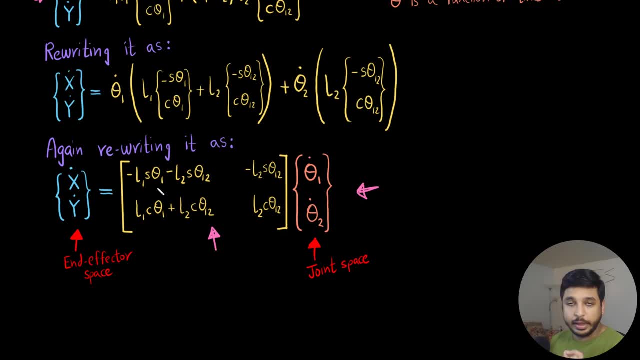 of time. so it depends on the value of theta 1 and theta 2. so if you were to change the configuration- that is, the position of a robot- this matrix would change. now there is a name given to this matrix and it is called the jacobian. 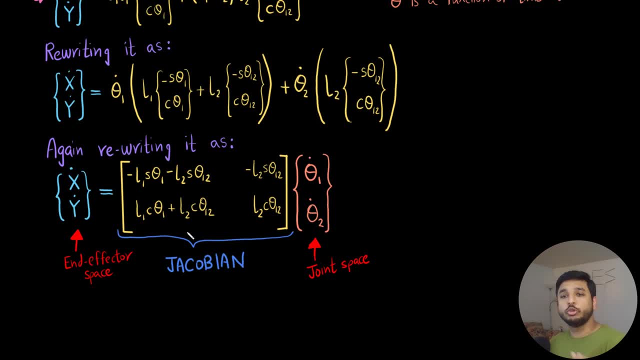 so this matrix right here, which in this case is a two cross, two matrix, is called the jacobian of a robot, and what it does is it just relates the joint space, which is this one, to the end effector space. another way to see it is: if i have the joint space here. 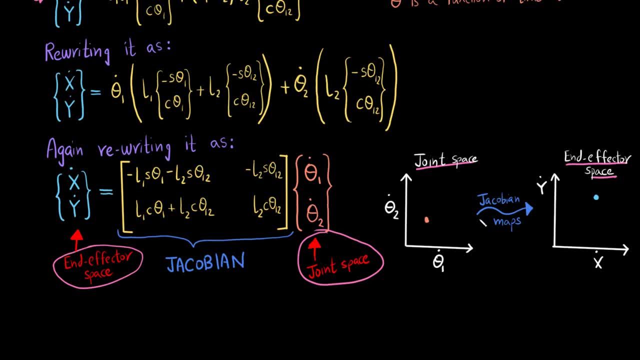 and i have the end effector space here. so the jacobian maps the joint space to the end effector space. so if you were to give me any value of theta 1 dot and theta 2 dot, i am just going to multiply that value by the jacobian and i would get. 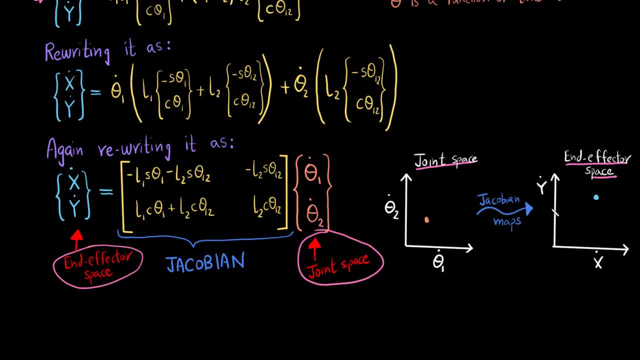 the, the x dot and y dot value, so the velocities of the end effector. so that is what the jacobian does, and if i just write this out compactly, i get this equation right here, which is a very important equation in robotics, which is: x dot equals to j times theta dot, where x dot. 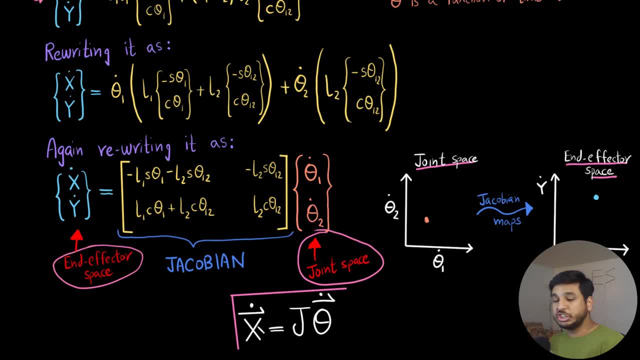 equals to the vector of my end effector velocity. j is the jacobian and theta dot is a vector of my joint angles. so let me just highlight this. so this equation right here is a very important equation in robotics, which just tells you that the jacobian maps the joint